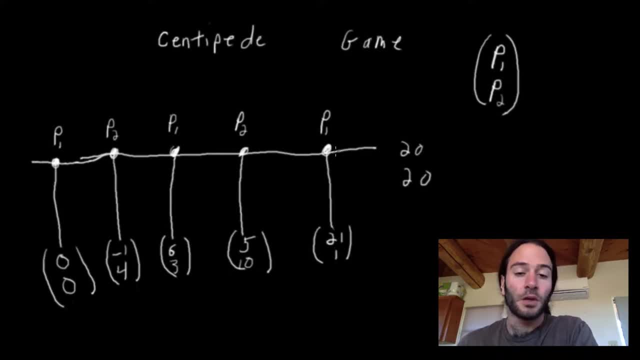 21, and player two gets a payoff of one. If he chooses to keep going, the game ends and they both get a payoff of 20.. So we see that if they both choose to keep going the whole way through, they both get a payoff of 20.. And if they both choose to keep going, they 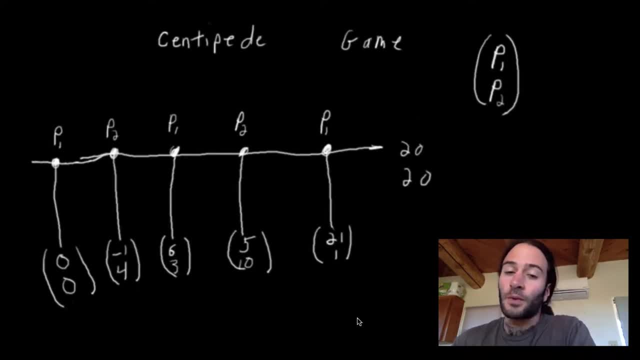 both get a payoff of 20.. What we're going to see, unfortunately, is that this under full rationality assumptions- I'm ruining the punchline here- but this will never happen, And we're going to see this through backwards induction. So let's suppose we're player one. 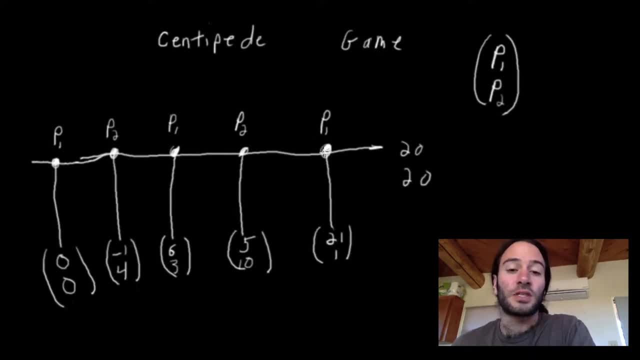 and he got all the way here. Does he choose to stop or to keep going? Well, if he keeps going, he gets a payoff of 20, but if he chooses to stop, he gets a payoff of 21.. So that one. 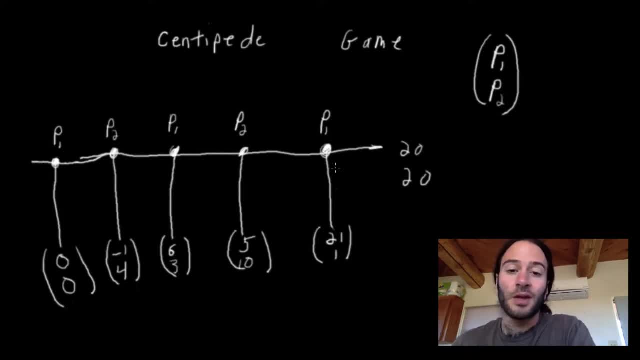 is going to get a payoff of 21.. And if he chooses to stop, he gets a payoff of 21.. So if player one gets here, he's going to stop. So what I'm going to do here is I'm going to write. 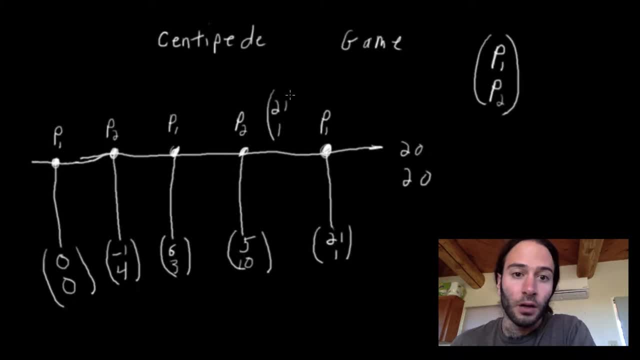 21,. 1 up here. And what this represents now is what happens to player two if it were to choose to keep going, knowing that player one will stop because it's in player one's best interest to stop. So now we go here and we say: okay, player two, are you going? 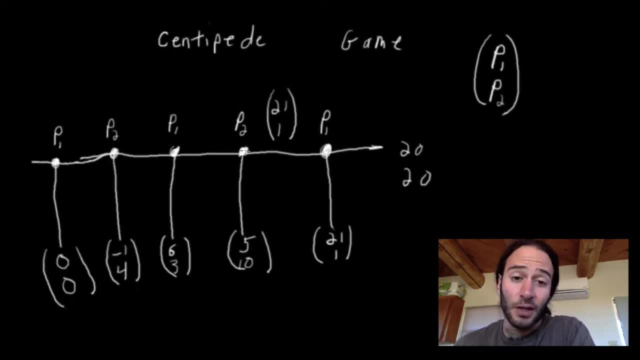 to stop or keep going. Well, if he keeps going, he only gets a payoff of one, because he knows player one will choose stop, But if player two chooses to stop, he'll get a payoff of 10.. So player two will choose. 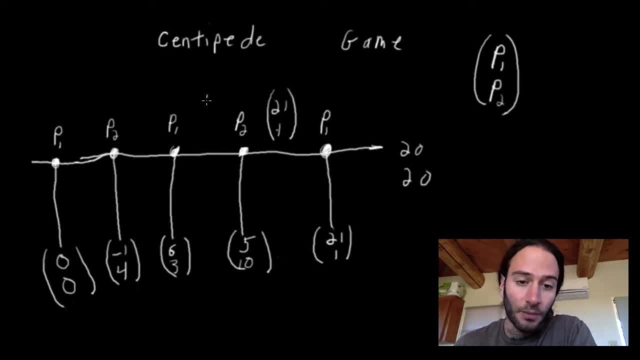 stop because 10 is better than one. So I'm going to put up here the 5 and the 10. And we repeat the same thing for player one. If player one gets here and it chooses to keep going, player two will choose to stop, And what that means is that it knows that if it. 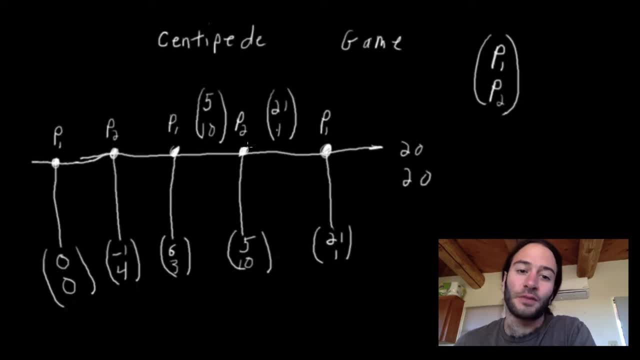 keeps going, player two is going to stop because he knows that if he chooses to keep going he will only get a payoff of one. So we'll put here that player one is considering the value of 5 to keep going, or the value of 6, the payoff of six to stop, Since six. 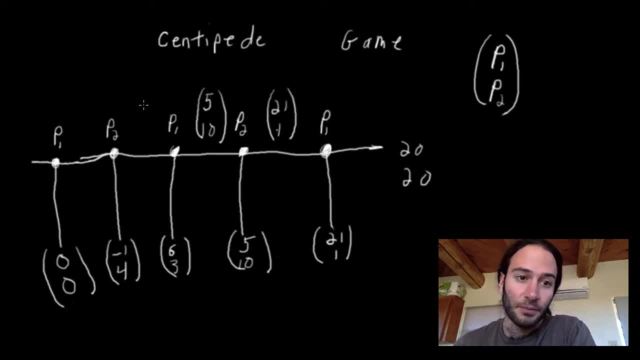 is greater than 5, player one will choose to stop, So I'll write the payoffs here again. and now player two has another decision: If it chooses to keep going. he chooses to keep going, which is located where paying off forms is Now.